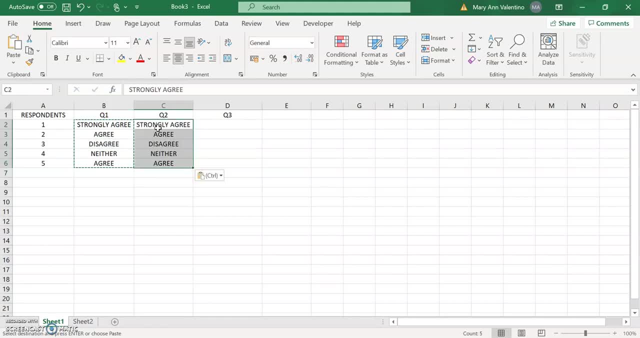 copy this, Then I am going to change the answer here. For example, this is agree And this is agree And this is neither. Okay, Then let us copy again. So let me go back the answer of strongly agree And for example, this is: 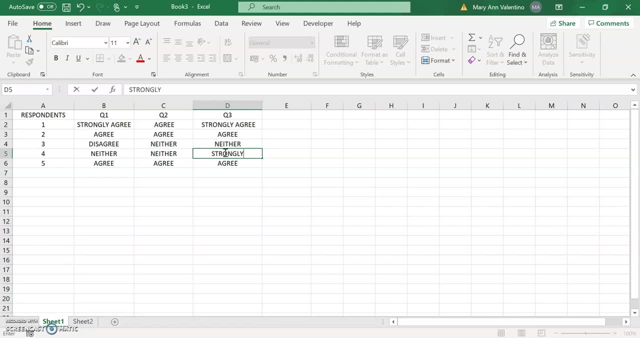 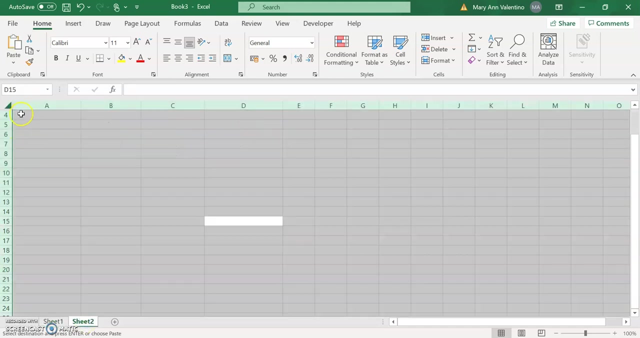 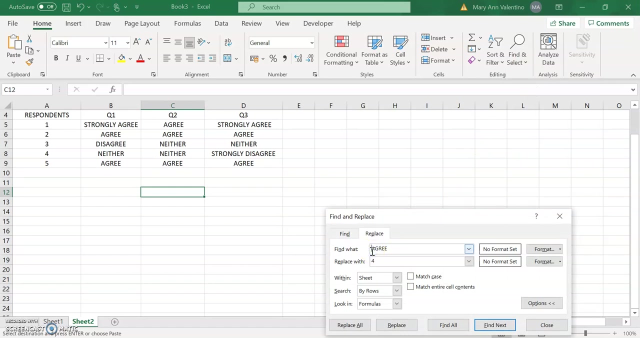 strongly, strongly disagree. Okay, So, after typing here the answer of the respondents, So copy this excel and then paste it with your sheet. okay, now replace all the answer of your respondents into value. so what are you going to do is click the replace and then type here on the find one. 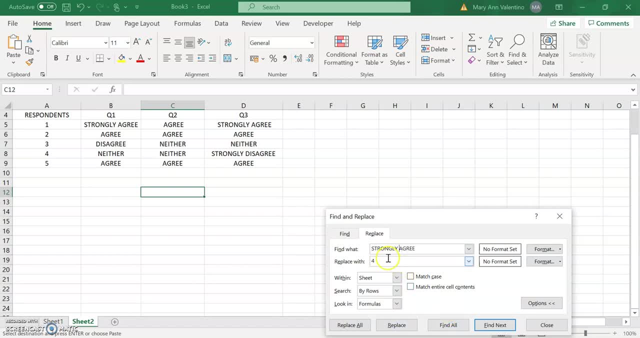 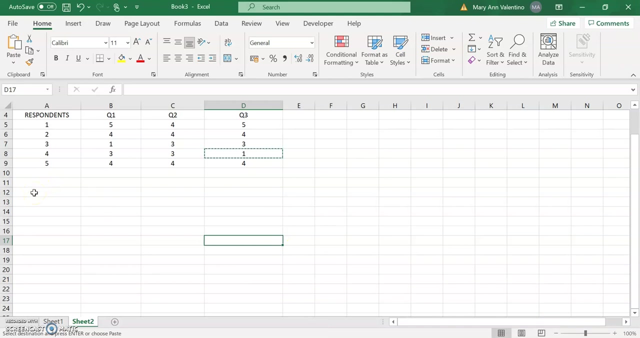 then replace it with a five, then look what will happen, okay. and then for the agree, so the value is four. then for neither, the value is three, okay. then for disagree, which is two, then strongly disagree, which is one- okay, oops, what happened here? strongly, okay, strongly disagree. so what replace? okay. then, after changing the value, here is: 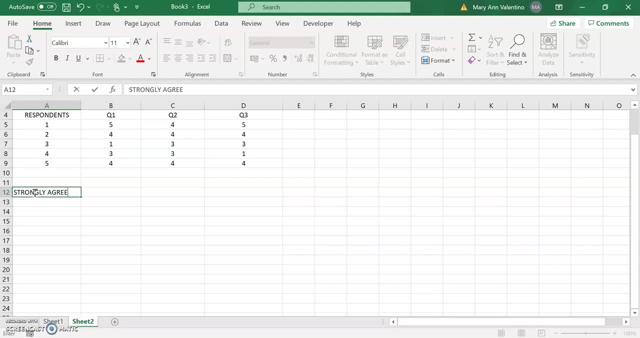 let me type again your category, which is strongly agree, agree, either disagree and strongly strongly disagree. now let us calculate how many respondents are going to be in this category. now let us calculate how many respondents are going to be in this category. respondents answered strongly agree in question one. okay, so let's have a formula which is equal. 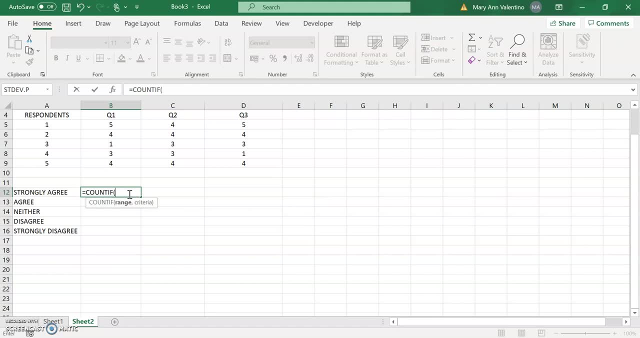 column if and then select the cell, so from d5 to respondents five, and then what is the value for strongly agree, which is five, then those parentheses then enter. press enter on your keyboard so how many respondents answer strongly agree, which is one. only then let's copy the formula here, but first let us have here a dollar sign. 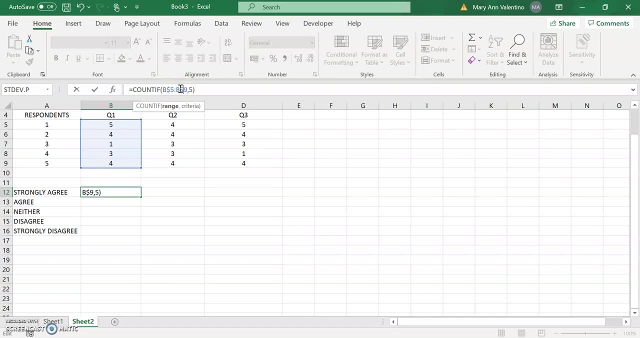 so that it will not be change the cell. so let's touch here and then change the value into four. okay, and then three. so for the disagree, which is two, and this is one, so Okay. so how many respondents answered strongly agree in question one, So we have one. 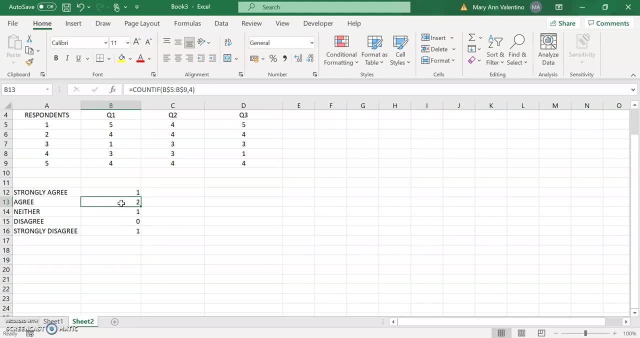 How many respondents answered agree in question one: We have two. Okay, one, two. Then how many respondents answered neither in question one, So we have one. And then how many respondents answered disagree in question one? So there is no one answered disagree. 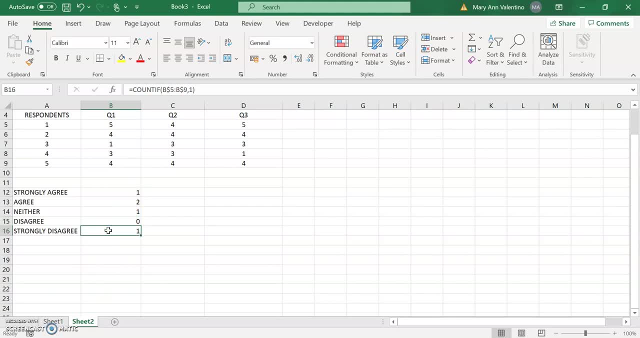 then how many respondents answered strongly disagree in question? one, so we have one. so let's say, uh, you change the answer uh respondents five into five, as you can see, the value of how many respondents did answer uh strongly agree will change. okay, so it changed into two. so we have uh. two respondents answered strongly agree. 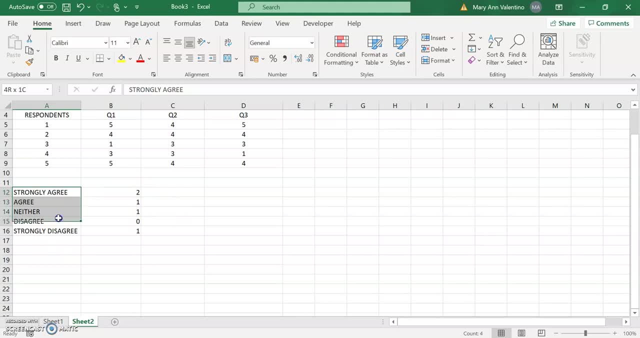 now how we will pull percentage here. okay, so let's let me copy again the category. okay, so let's have here percentage for uh. two respondents answered strongly agree. so for this let us have equal. and then uh, select the cell and then divide how many respondents answered on your serving, so we have five and then close five to six, then press enter. 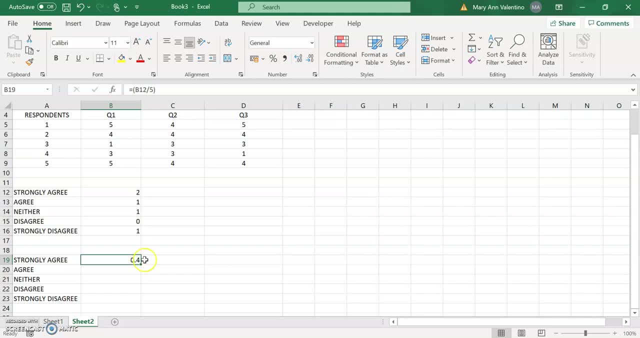 then for a order you to have percentage here. so on your menu or on your standard toolbar, click the percentage and then, as you can see, change into 40 percent. then stretch the cell into strongly agree. then it will, uh, change it into how many percentage percentage, how many respondents percentage, and answered strongly agree. then agree neither. 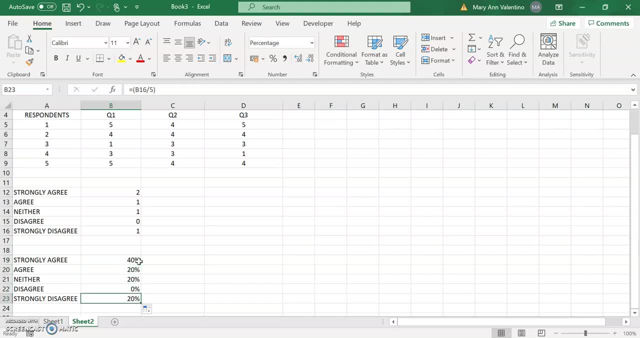 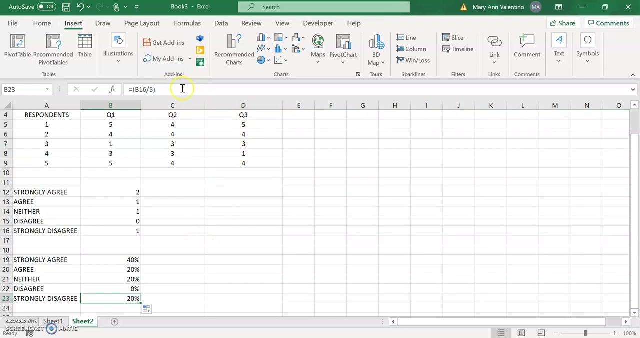 disagree and strongly agree. so it's very easy for you to use the excel in order for you to tabulate the uh survey results and to have a percentage in your excel. now let's have um a chart here, so clip insert. then let's have here a pie chart. okay, so a 3d pie chart. so since 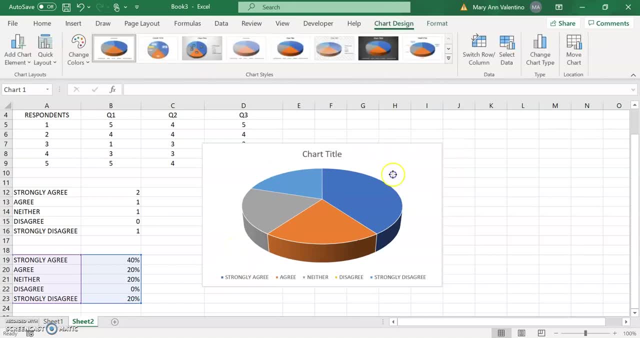 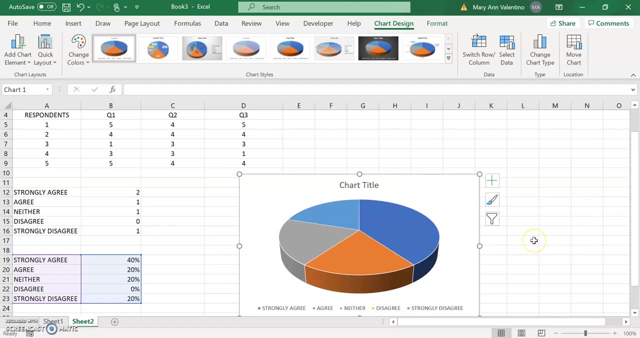 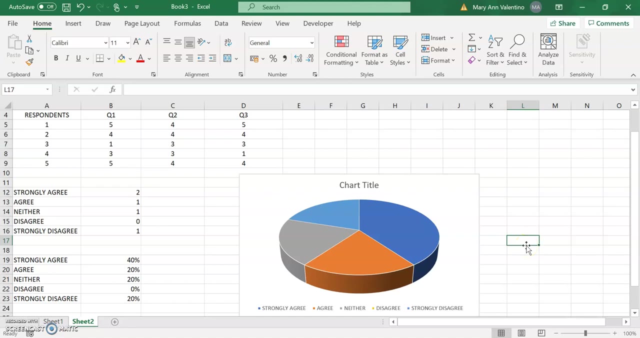 we choose the excel on the percentage automatic, you will have a chart for your uh survey results, so i hope that you learnt it will in this video, the topic. by the way, you have nice time with me, so i hope you learned something new on my video lesson. don't forget to subscribe. 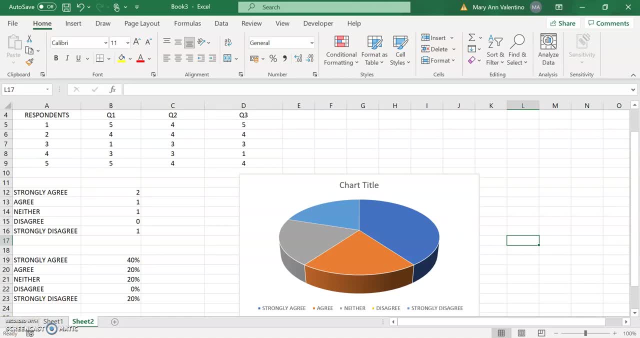 like and share. thank you and god bless.